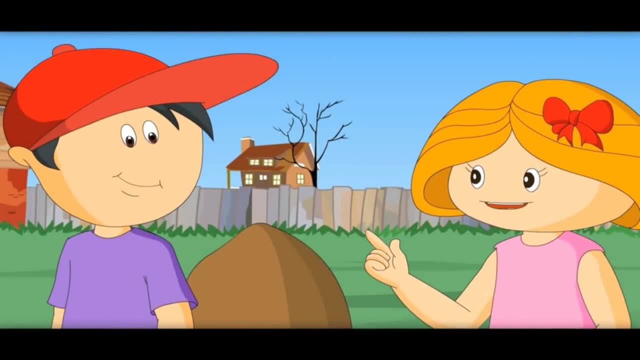 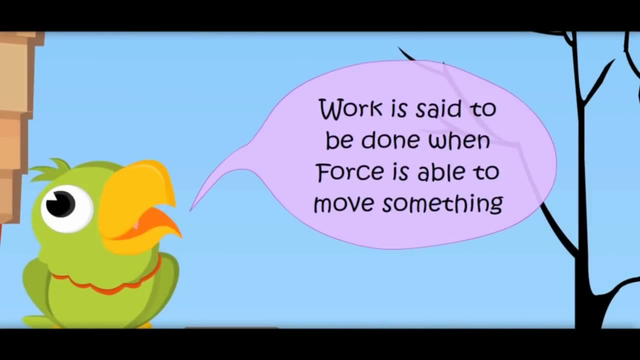 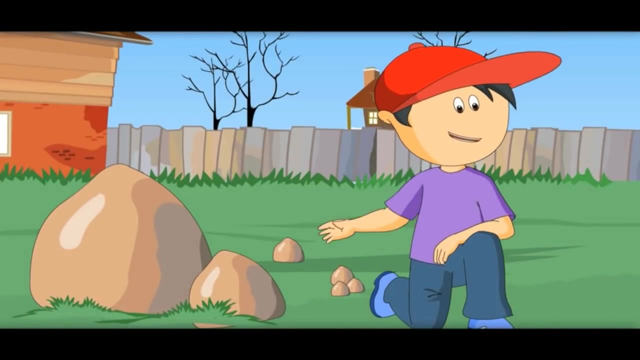 Why, Whatever force you apply, but if things do not move, that means work is not done. Ah ah, work is said to be done when force is able to move something. Oh. so let me leave this big stone, Let me pick these smaller ones. 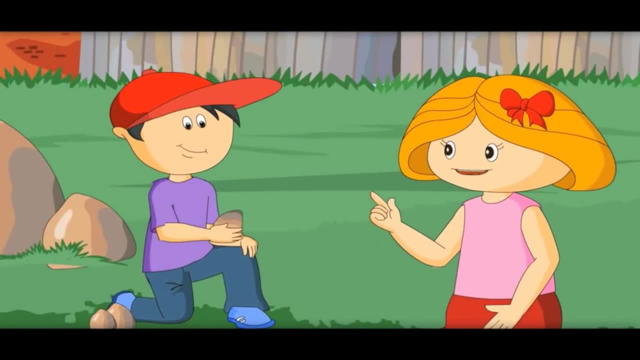 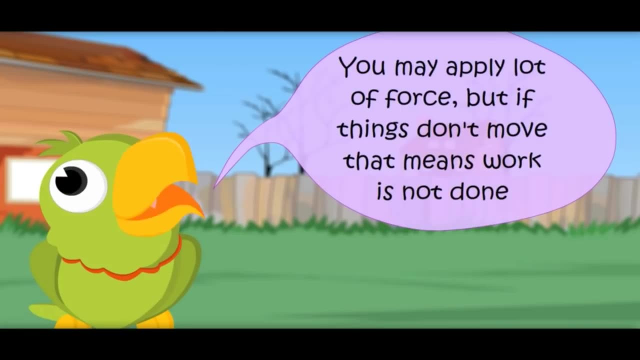 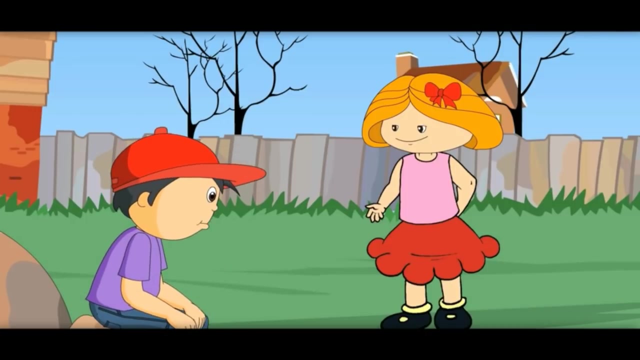 Yeah, this is the right choice. At least you are moving few things and some work is being done. Ah, ah, you may apply lot of force, but if things don't move, that means work is not done. Oh, I don't have energy to work, I don't have ability to work, I am tired. 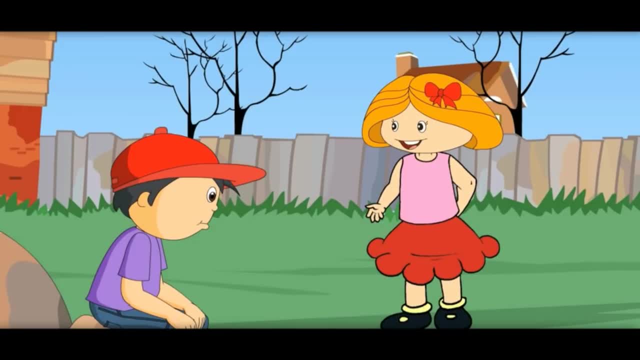 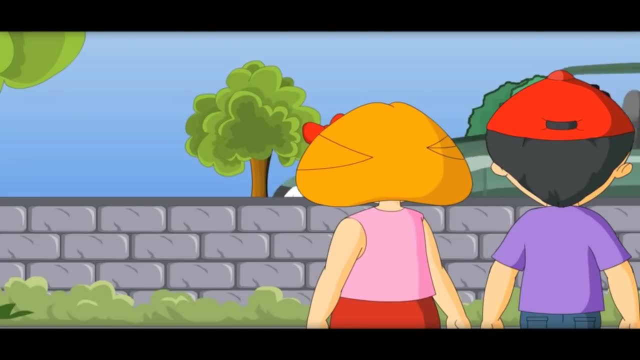 Yes, you are right, Energy is not enough. I don't have energy to work, I don't have ability to work, I am tired. Energy is ability to work, Ah ah. energy is ability to do some work. Do cars also use energy? 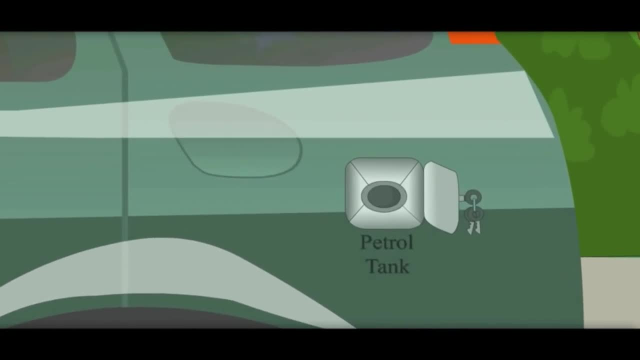 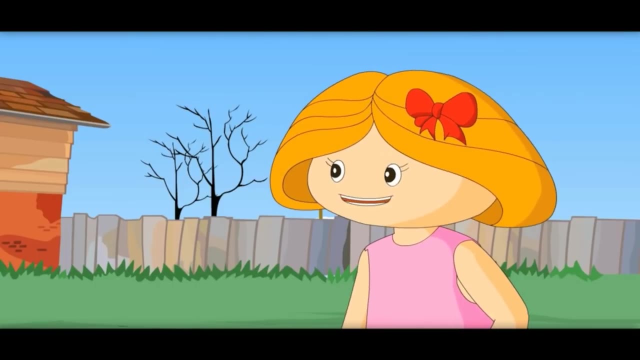 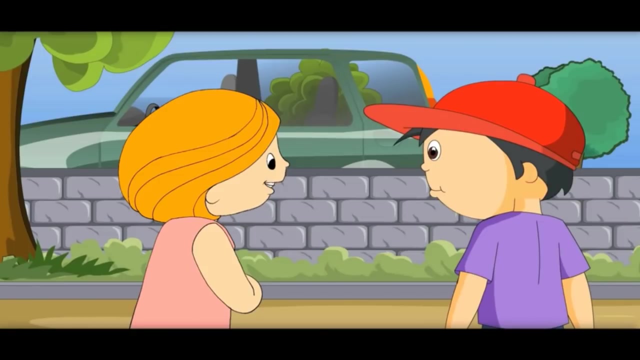 Yes, they use petrol or gas as energy. So petrol or gas has energy which make things to move. All things require energy to move. So we can store energy. Yes, energy can be stored, Like in the petrol tank of a car. 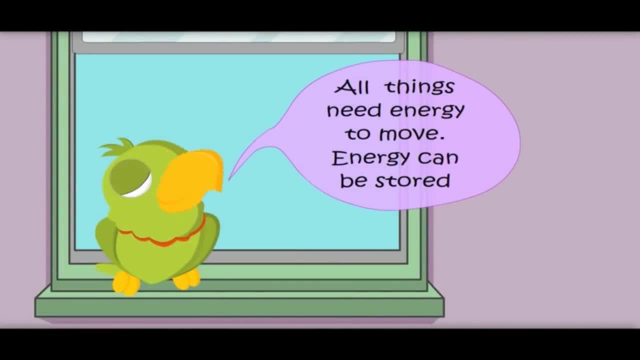 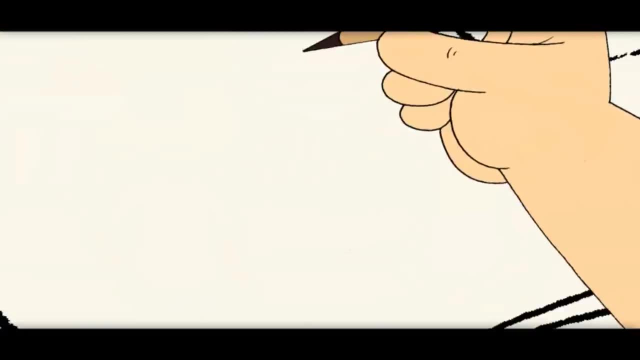 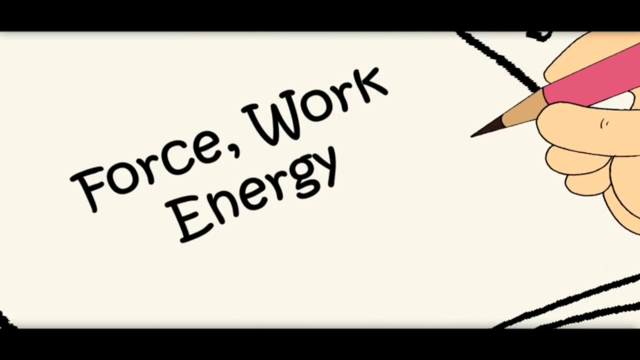 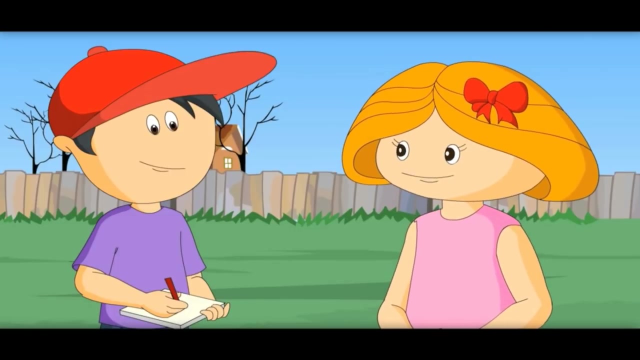 Ah, ah. all things need energy to move. Energy can be stored. Oh, I used so much force and energy, but very less work was done. Yes, Jimmy, You applied lot of force and you used so much of your muscular energy, but you could only move few things. 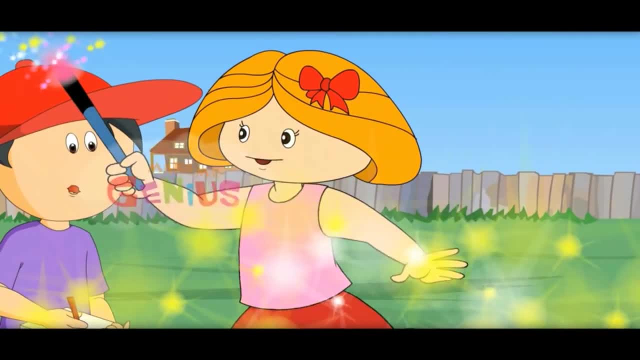 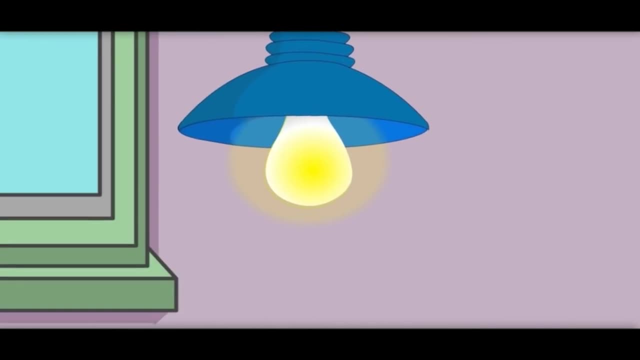 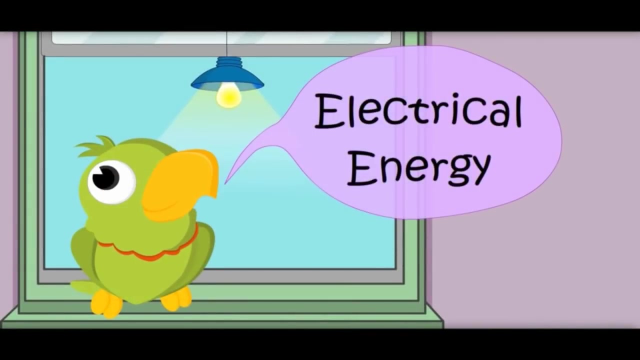 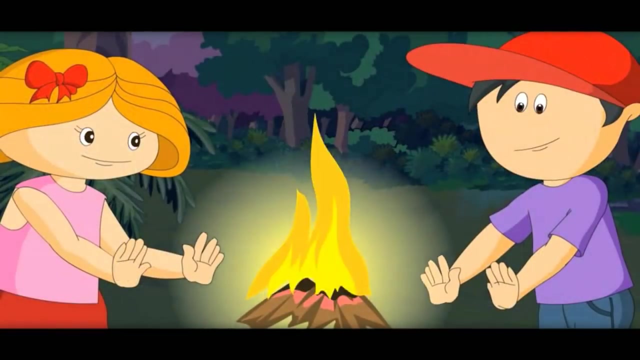 Hence less work was done. Now we would see different types of energy. Oh, this bulb is giving so much of light. Yeah, it works on electric energy. Ah, ah, electrical energy. Hey, this fire is giving so much of heat.